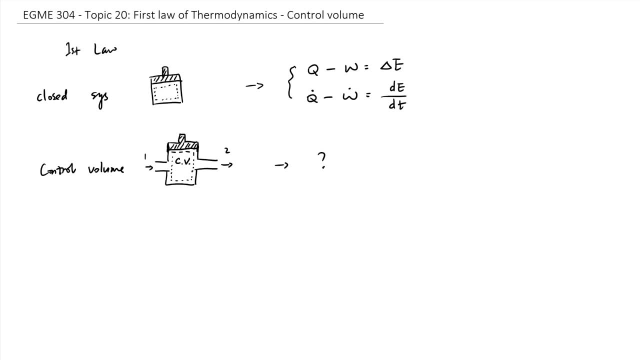 dot, that is power, and right-hand side becomes dE over dt. So our question is: what will this equation change into when we start dealing with a control volume where there is a inlet or an outlet or more than just one? We can start from the equation we already know for the closed system, which is Q- heat transfer. 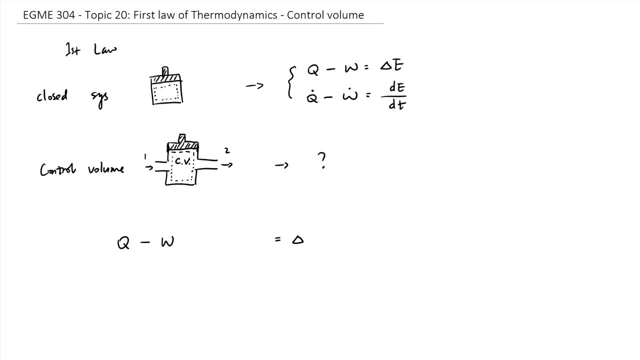 minus W. right-hand side is delta E, Because even when we move on to the control volume, we will still have to deal with heat transfer, we will still have to deal with work and then there will still be the change of total energy as shown on the right-hand side. But what has changed is 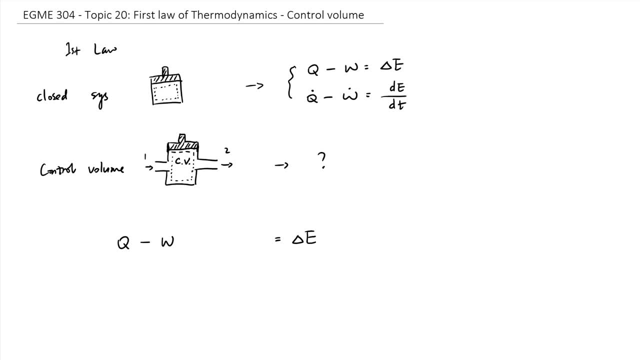 volume. you have an inlet and an outlet. at the inlet mass keeps coming in. when mass comes in it brings in energy, so we need to add the amount of energy brought in at the inlet, so plus capital, EI at the outlet. mass keeps leaving our system, so energy also leaves our system with the mass. so waiting to subtract the 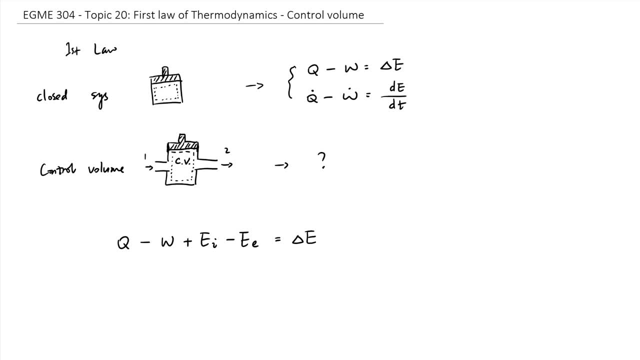 amount of energy leaving from the exit. so we write down minus capital EE. so this is pretty much the equation for our control volume. but we're not at the final form of this equation yet. we need to rewrite this equation slightly. so first thing we do is to rewrite those two big E's: Q minus W plus capital EI. 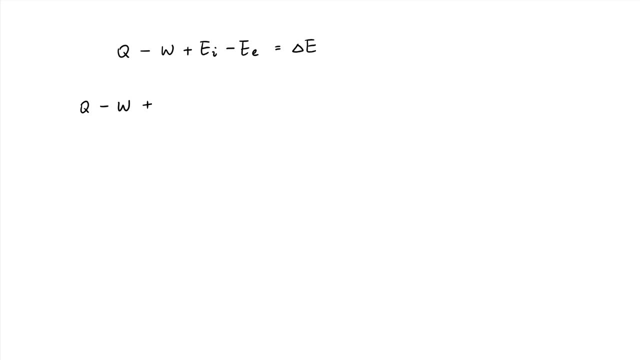 capital. E stands for total energy and we know total energy has three components. they are kinetic energy, so 1 over 2 m VI squared, plus potential energy. potential energy is mgz and I give it a subscript to indicate this is at inlet mi and a zi and then 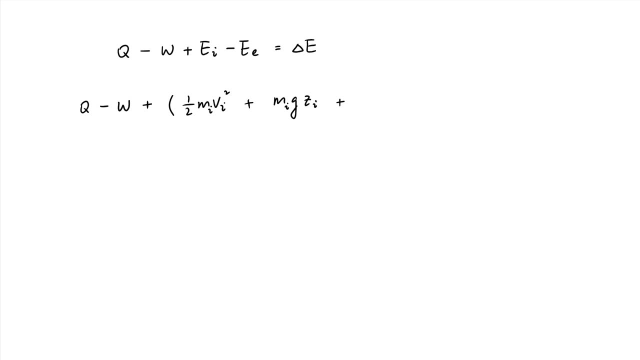 the third component within total energy is internal energy. internal energy is equal to mass times specific internal energy and again we give it a subscript to indicate this is the inlet and then we just need to repeat for EE the sign before it is minus and the capital EE. 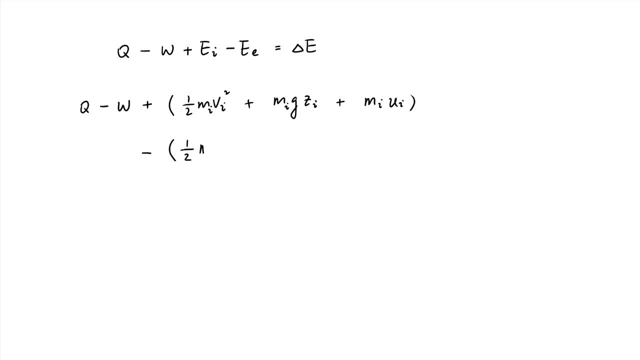 will just be the same thing: 1 over 2 me ve squared plus me g ze plus m e u e, and the right hand side will be Delta II. next, what we do is to divide every single term by time. if we do that, Q becomes Q dot and W becomes W dot. and 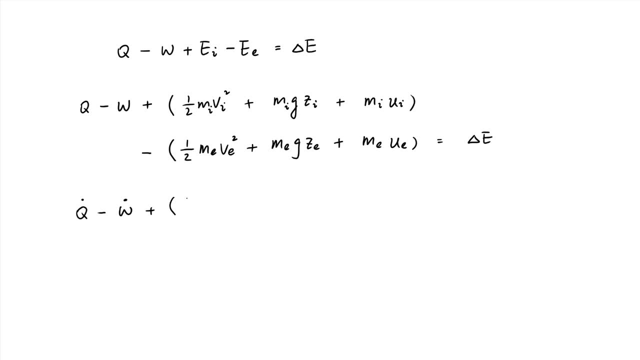 everything inside the parenthesis becomes 1 over 2. mass over time becomes mass flow rate at the top, with the dot on top of it, and same thing happens to the two remaining terms: m dot I G zi plus m dot I you I. same thing happens to the exit right hand side becomes derivative. 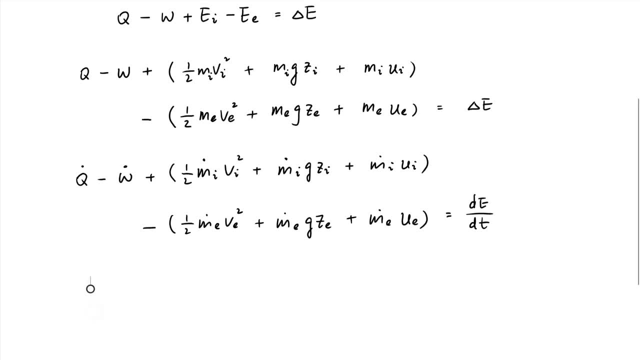 capital E over DT. so now we're at a step closer to the final solution and the next we just need to focus on discussing. what is this W dot? What is this W dot? Let's quickly sketch our diagram again. We have a piston-cylinder assembly. 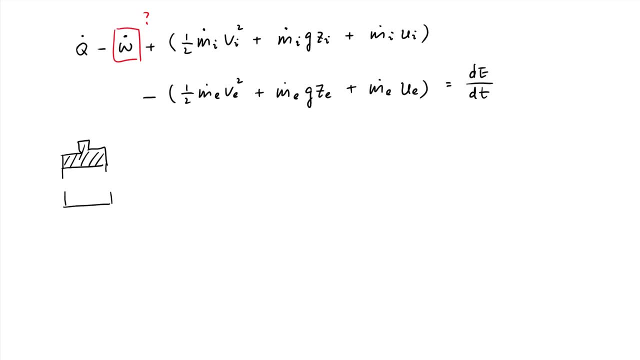 but this time we have an inlet and outlet, unlike before. We choose everything within the cylinder as our system and obviously this is a control volume, because you have an inlet and outlet. Inlet, we call number one, and outlet, we call number two. 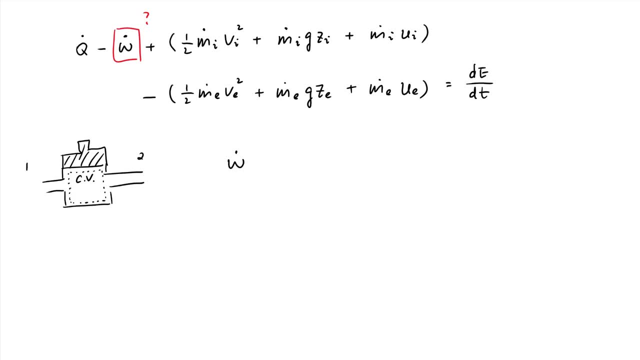 Okay, so now, what is this W for our whole system? So this W? first of all, the piston will still be able to move up or down, which we call WCV. This term comes from the moving parts. In this case, the piston moves up and down. 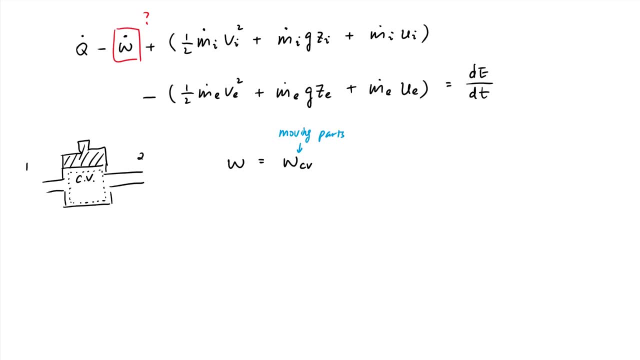 so it's going to contribute to what Work. However, what is different is now we also have to take into consideration the inlet and the outlet, because at the inlet what is happening is the pressure is pushing the fluid into the control volume to push something over a distance that is work. 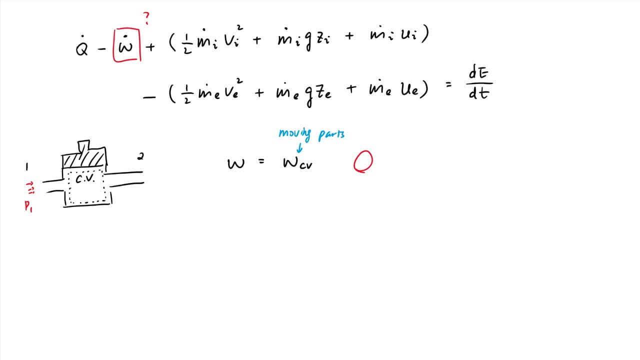 So we need to add one more term to account for the work happening at the inlet. And then same thing happens at the outlet. At the outlet, the pressure pushes the fluid out of the control volume and again to push something over a distance that is work. 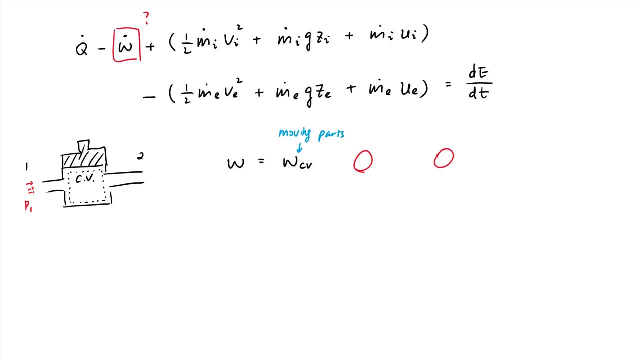 So we need to add one more term to account for the work at the exit. Okay, so now let's start from the inlet. We know work is force multiplied by distance, and the force is F, distance is D. However, force can be written as the force multiplied by distance. 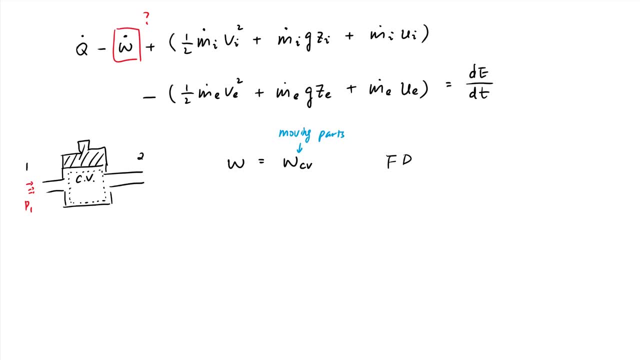 written to pressure multiplied by area. So we're going to change force to pressure multiplied by area And now let's give it a subscript to indicate this is the inlet. PI, which is the pressure of the inlet. AI is the cross-sectional area of the inlet. So this cross-sectional area, 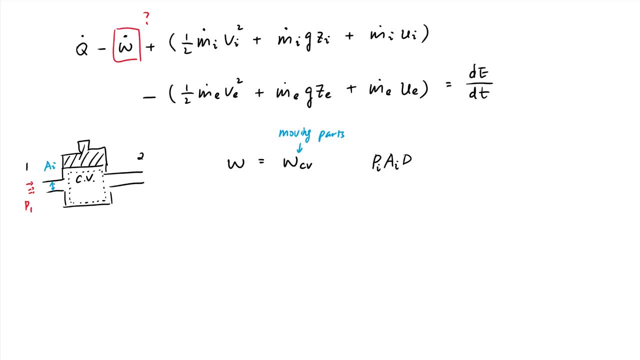 is my AI And D is the distance. We call it DI. And now let's determine the sign before this term. Should it be plus or should it be minus At inlet? what is happening is you are pushing the control volume and you are pushing my system. Therefore, my system gets pushed. If my system gets pushed. 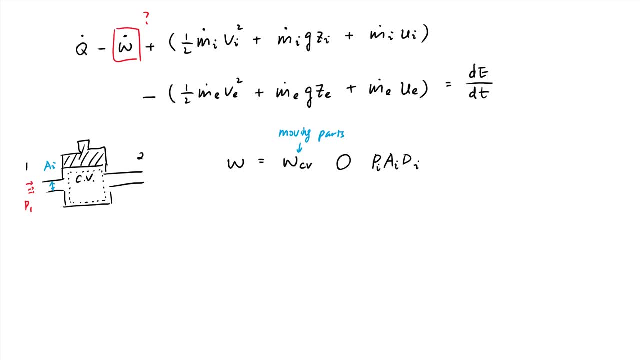 that means my system consumes water. If a system consumes work, the work must be negative, And same thing happens to the outlet. At the outlet, the term would just be PAD again. But this time everything is at the exit, So give. 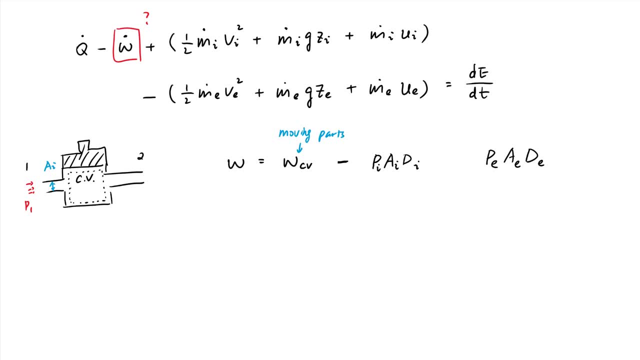 it a subscript E, And now we just need to determine what is the sign before that. What is happening at the exit is my control volume is pushing the fluid out of it. So if my control volume the system pushes, then my control volume is the one to generate. 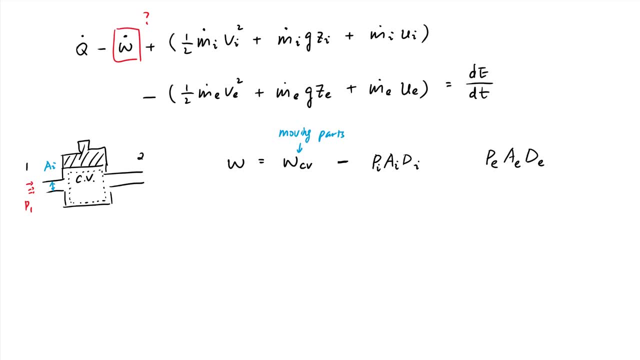 work. If the system generates work, the sign must be plus. So now we have accounted for all three sources of work for our W And if you take a look at the equation on top of the screen, in the red box, what we need is W. However, what we have right? 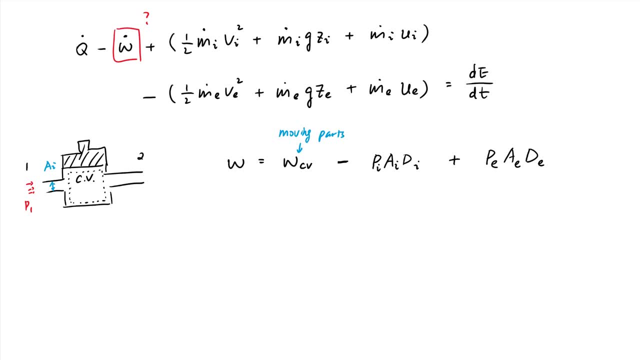 now is W. That means we just need to simply divide every single term by 2.. So people pushing the system. my control volume is the one to generate work, As you can see on the double eight. If the system generates work, the sign must be plus. 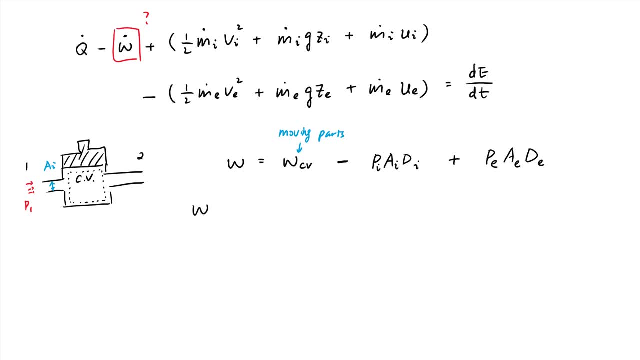 So if E is the least plus done on that wave in the bottom action cycle, D. So if E is the least, Then if the coinedices are at the exit and the working source is D time, w over time is w dot and in the right hand side wcv over time will be called w dot, cv and 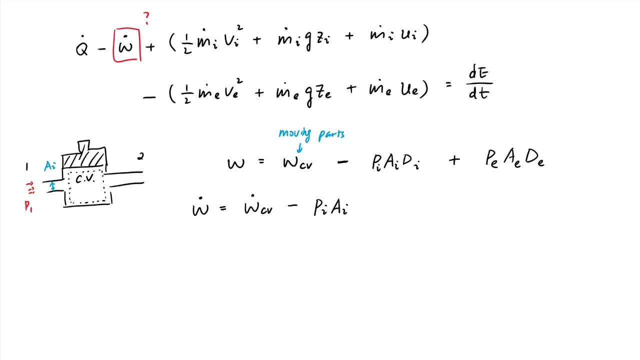 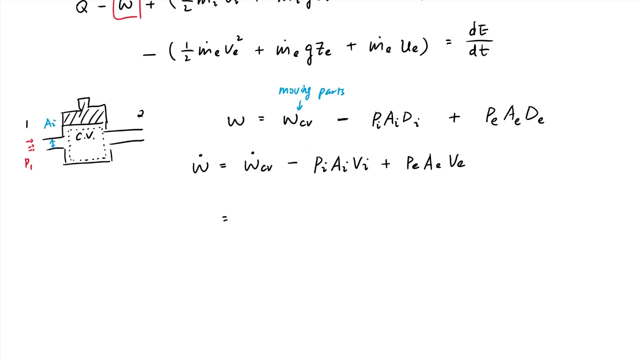 minus pi, ai, d is distance. what is distance over time? distance over time is velocity. so we write vi. so same thing happens to the third term in the right hand side: pe, ae and ve. ve is the velocity of the fluid at the exit. okay, next, what we do is a mathematical manipulation to the two terms in the 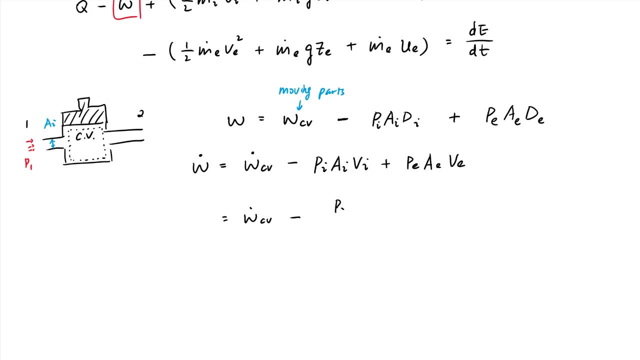 right hand side. what we do is, first of all, we have pi, ai and vi, and what we do is to multiply this whole term with density and then divided by density, so e cosine is still true. then we do the same thing for the last term in the right hand side: pe, ae and ve, multiplied by density at the exit, divided by density at. 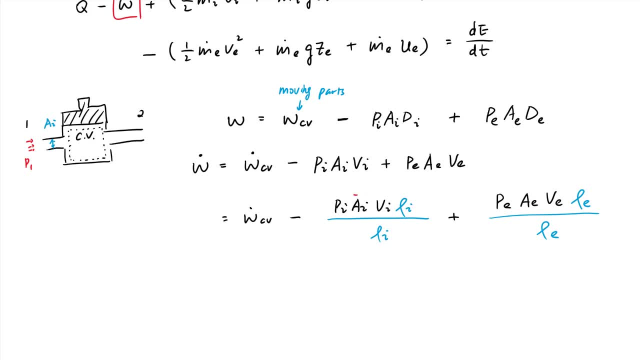 the exit. the reason we do that is rho va. rho va is something different. rho va is equal to the definition of mass flow rate, so this equation can be simplified and, in addition, what we can do is density. density is the inverse of specific volume, so we can rewrite both denominators into specific. 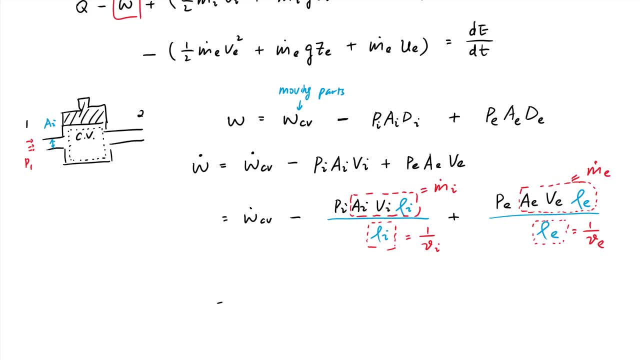 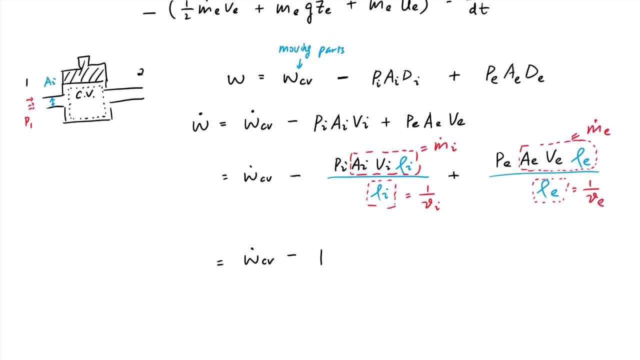 volume new. now this equation will be changed to w dot cv minus PMI times M, that i times nu. i 3 term will become PE and e times Newy. so now, finally, we have reread and w tuat 3.. COME FROM THE BUILDING.